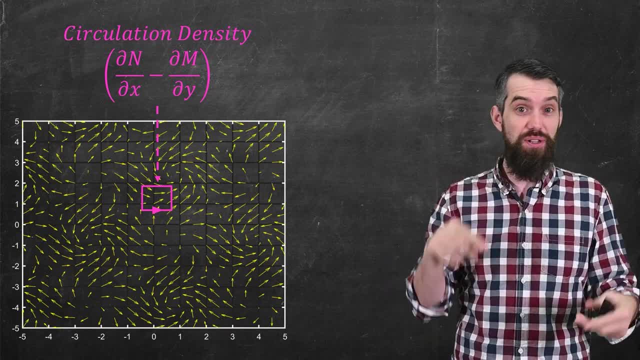 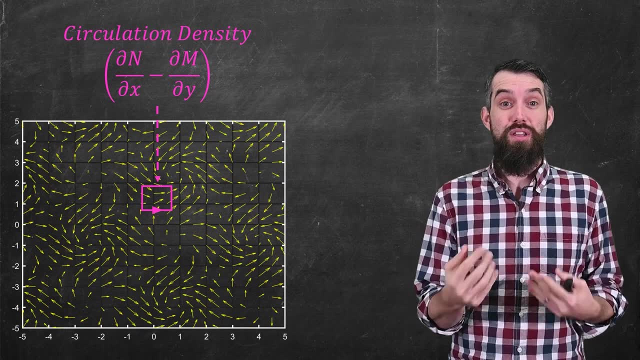 about this is that if I'm imagining my vector field as, say, a velocity field and some particles moving around in it, So what I'm doing when I take the circulation around this very small loop is I'm basically trying to measure the degree to which the vector field is moving around in it. 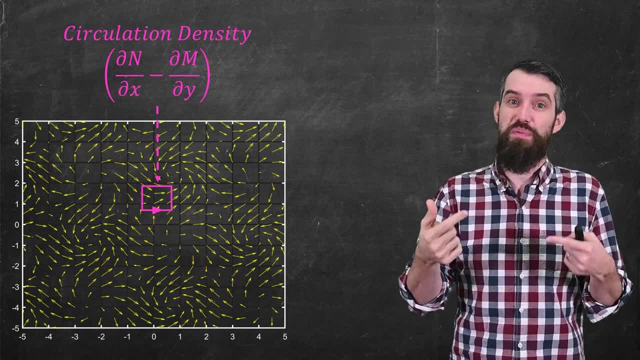 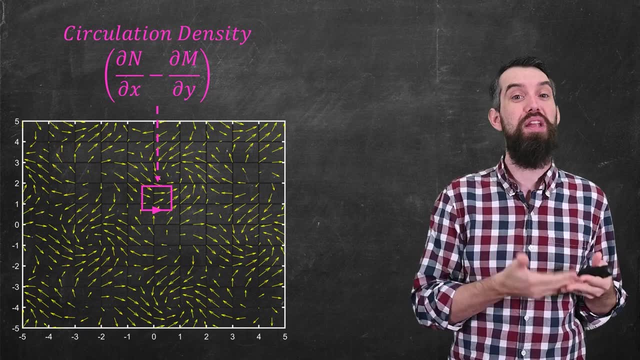 Where does this vector field go? Well, the vector field is curling at that particular point in the limit, as this loop gets smaller and smaller, And this is why we're going to call this a part of the larger thing called curl. So curl is the three-dimensional analog of this two-dimensional 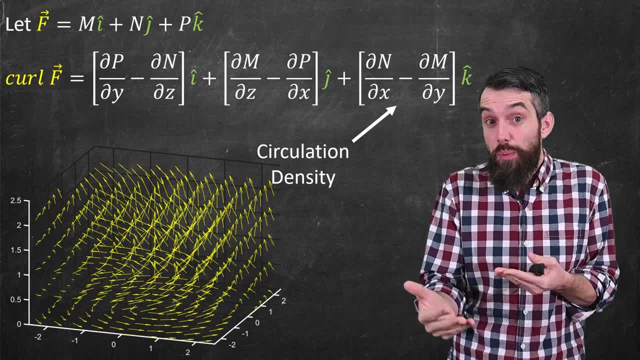 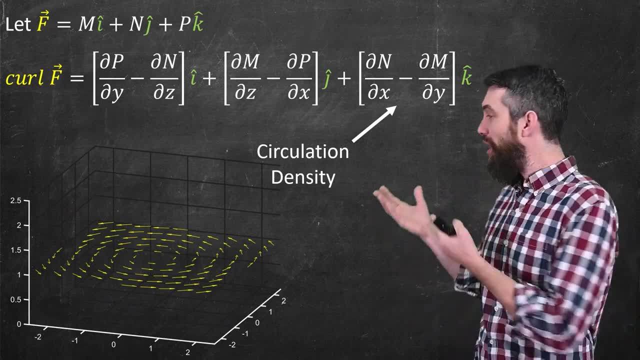 circulation density. So, returning back to our definition with the three different components, one other way to interpret the third component is: let me just imagine I'm just going to do a slice, a slice parallel to the xy-plane, ignored what their third component is, what their k-hat component is. I've just sort of leveled them. 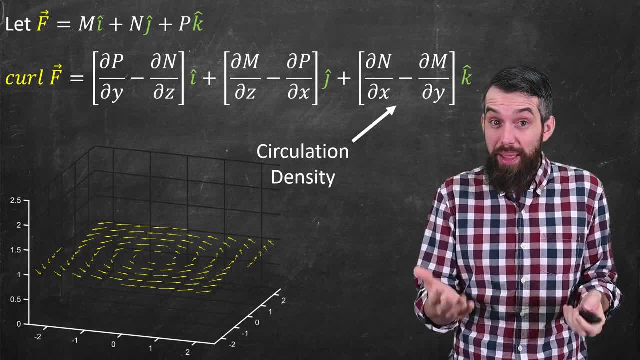 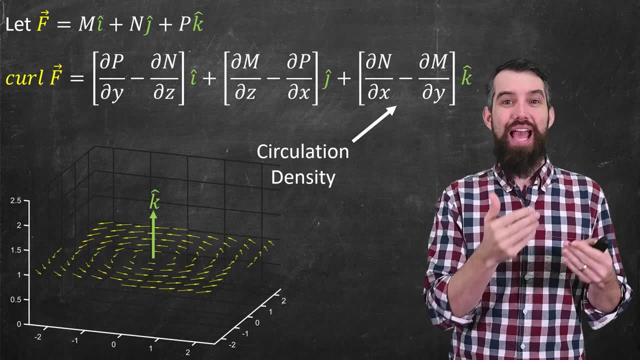 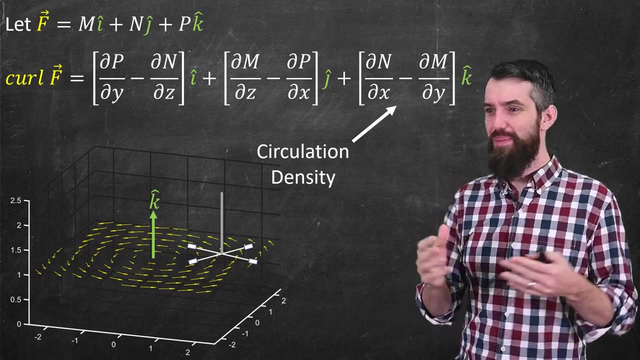 all off. Indeed, if I take a slice parallel to the xy-plane, then I would get some normal vector to that xy-plane, which I can call the k-hat vector. So what I have at this point is that the vector field is causing this curling in this plane that's parallel to the xy-plane. I'm going to put up a. 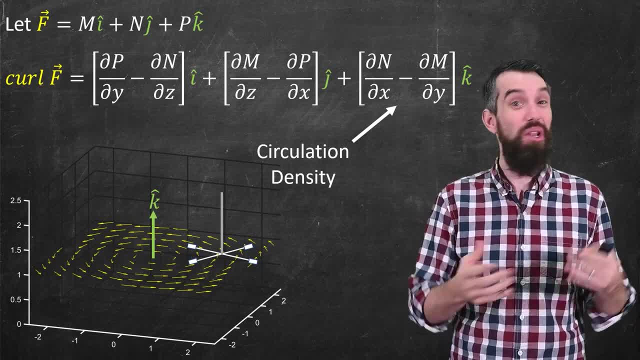 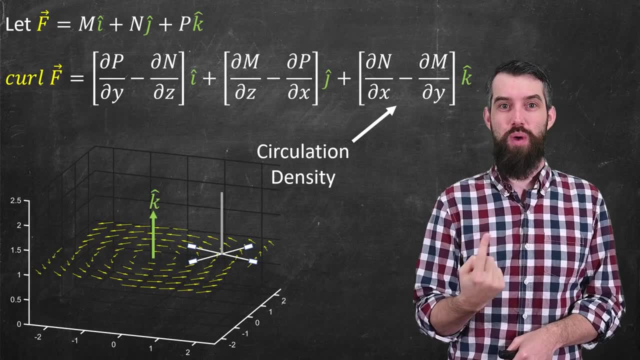 little spinner here. I don't know if this is clear. What I'm trying to imagine is like a little paddle wheel. This paddle has a fixed axis here, parallel to the k-hat, and then it's allowed to freely spin parallel to the xy-plane, And so if you imagine taking this into some body of water, for example, 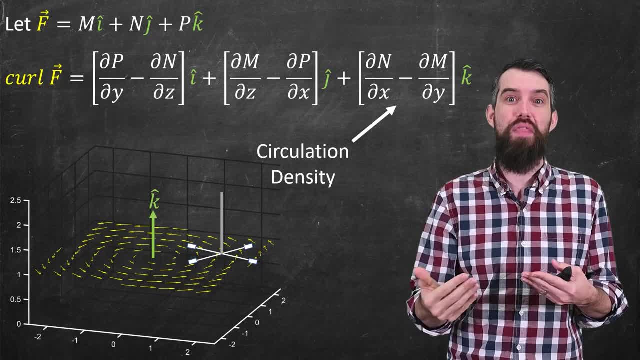 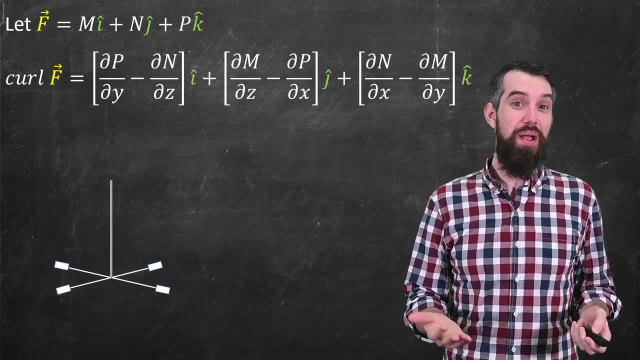 and you put this little spinner in, well, how much would it spin? That is what the third component, the k-hat component of this curl is representing. Likewise, if I have my spinner, which is pointing straight up, I could ask: well, my spinner pointed to the side, That is, my axis is parallel to the. 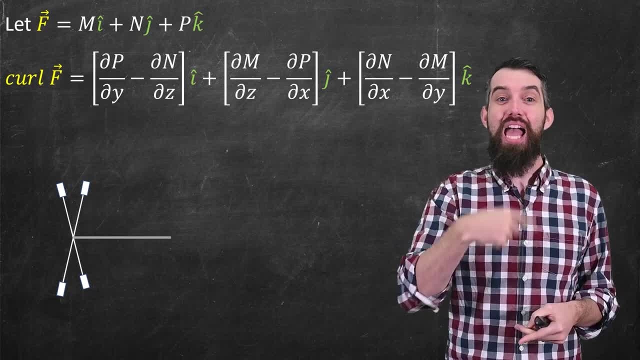 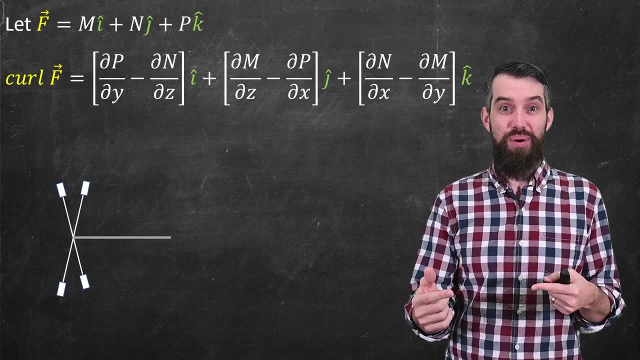 i-hat direction. so it's allowed to spin in the yz-plane. Well, that would represent the first component of the curl. how much spinning is allowed to happen there? And then in general, if I just take the spinner and I put it in the water and the only thing I 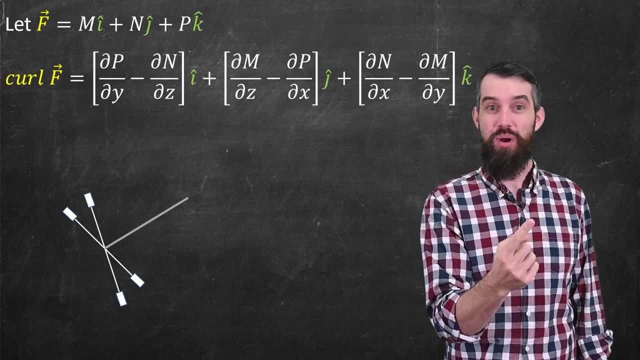 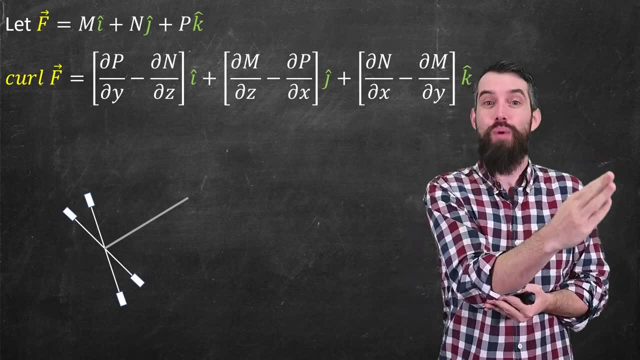 fix is that the actual point where it's at. so it's allowed to spin, but also the axis is allowed to point wherever. then what the spinner would do is it would end up fixing itself in some direction, depending on what the vector field was doing. It wasn't changing in time, It would fix itself and 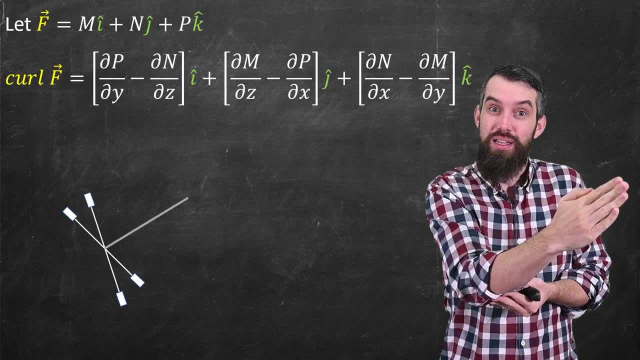 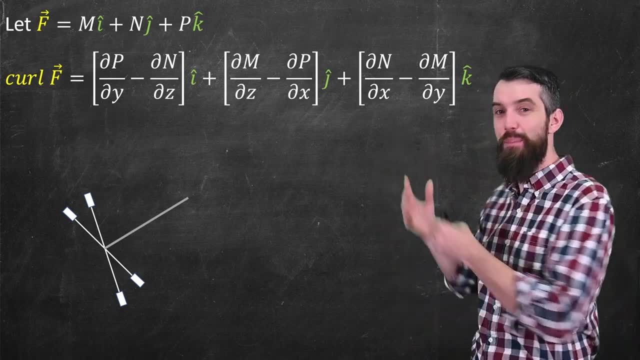 then it would spin around in that axis. Well, that axis is the curl. Okay, so that's a bit of a geometric interpretation of what curl is doing, but how do I actually compute it in a way that's a bit more sensible than this? 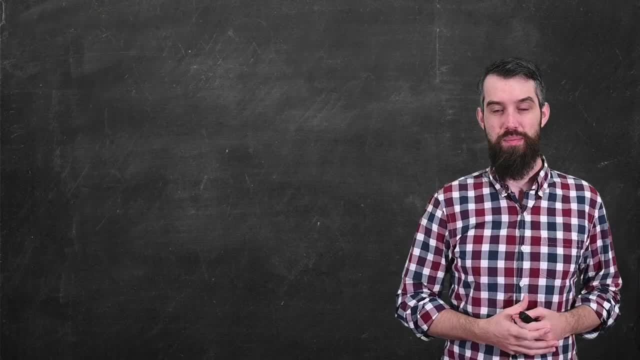 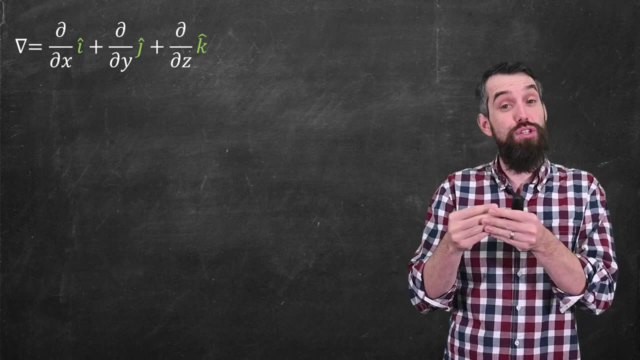 So I want to introduce you to the del symbol. This is shorthand for take the partial derivative with respect to x in the i-hat, plus the partial derivative with respect to y in the j-hat and the partial derivative with respect to z in the k-hat. 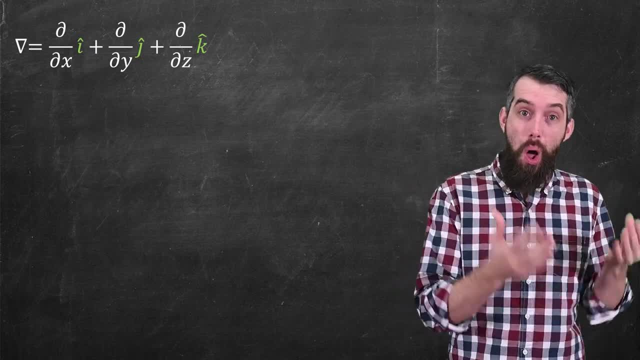 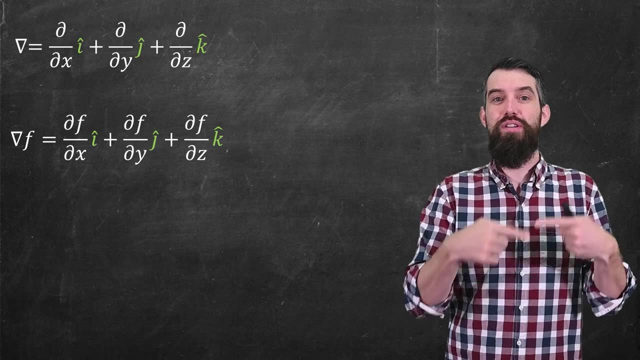 We've seen this before. We've seen this del operator before. For example, we've seen that the gradient of f del applied to f is the partial derivative of x with respect to x in the i-hat and f with respect to y in the j-hat and f with respect to z in the k-hat. 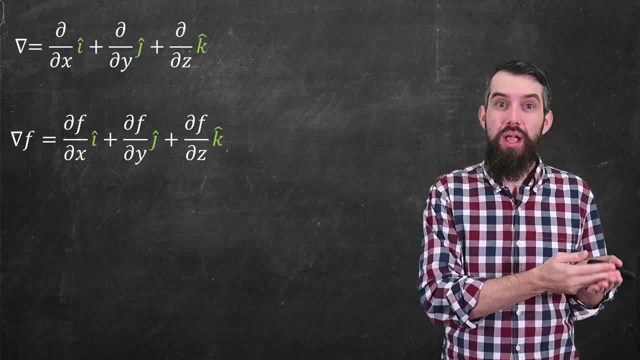 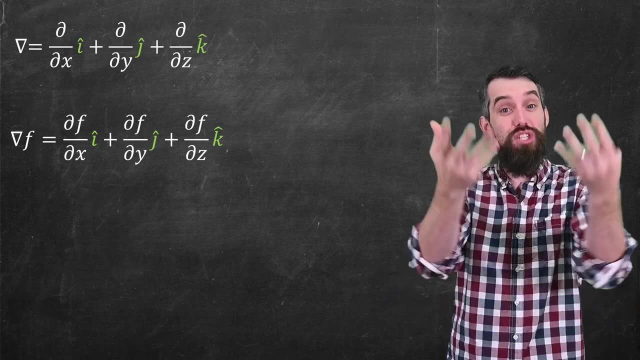 So what kind of object is del? Well, I said the word operator. An operator is something that takes some function and spits out another function. An operator eats functions and gives out other functions. So the del operator takes in the scalar function f and 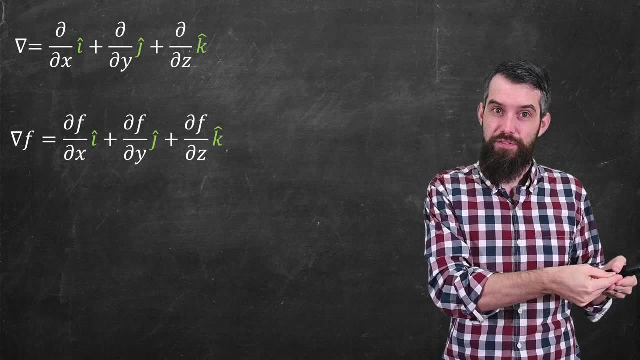 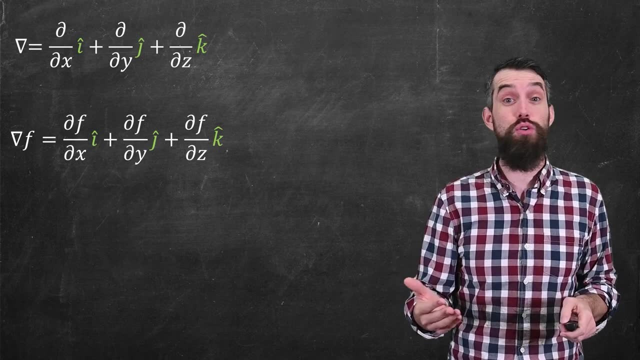 outputs the vector function gradient of f. Now, gradient of f here is only relevant because it's something we've seen in the past. Now going towards curl, here I'm going to do a completely different operation. This operation is what I'm going to call del cross f. 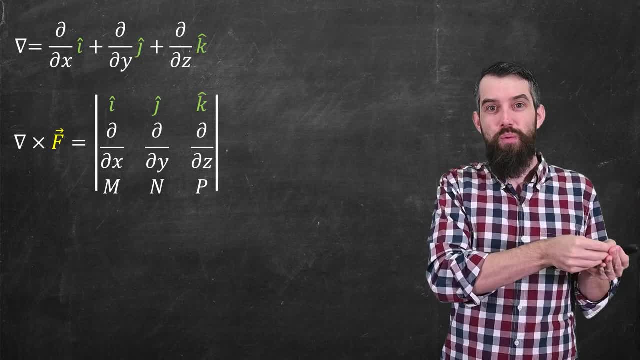 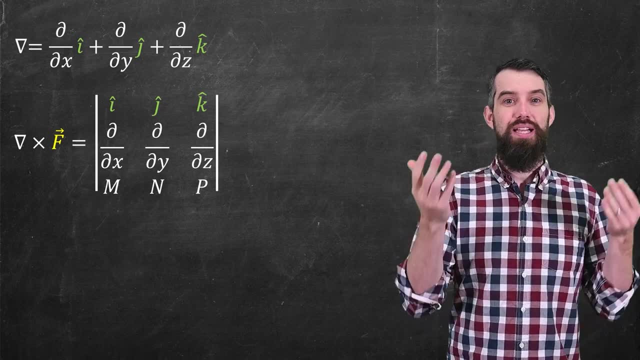 It is the cross product of this operator with the vector field f, And so I do my normal cross product trick of making a determinant i-hat, j-hat, k-hat in the first row. Second row is the first thing in the cross product which is partial respect to x, y and z respectively. 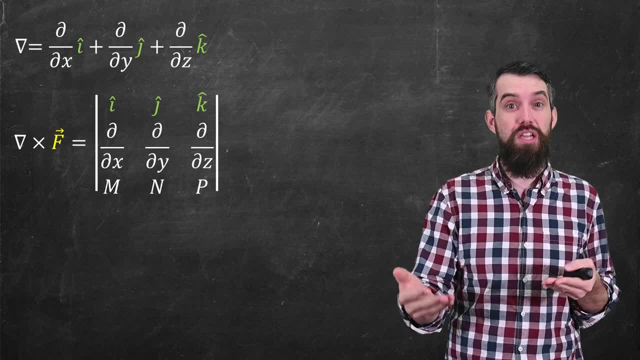 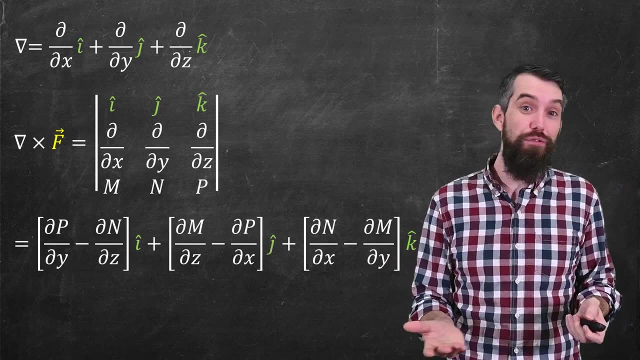 And then the three components of my field- m, n and p- go in the third row. Compute all of this out. It's just a cross product. And well, I get exactly what we had before, what we previously called the curl. 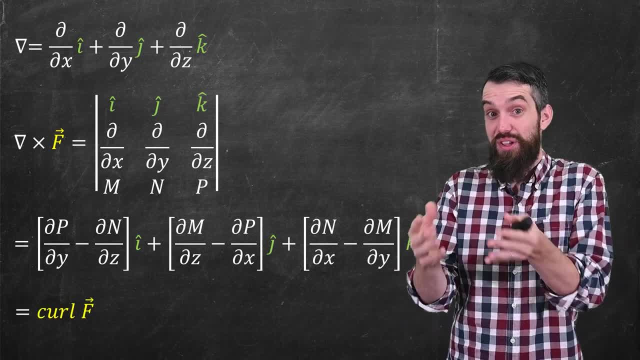 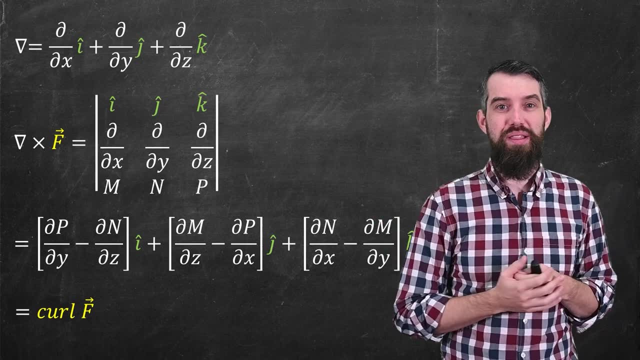 So now what this operator is doing is it's taking the vector field f and spitting out this new vector field, the curl of f, And so I often don't bother remembering this formula with the m's and the p's and the y's and the z's. 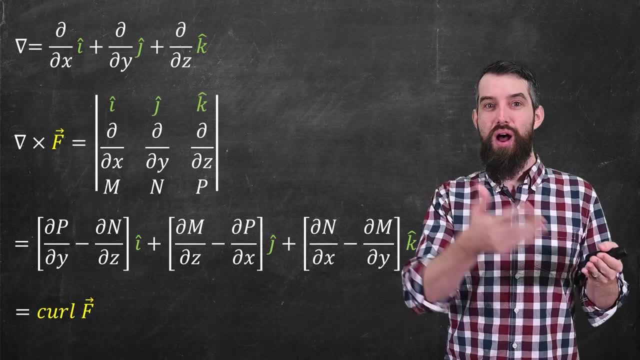 I mean you can, if you want to, it's totally fine. I just remember del cross f and I just compute out that determinant when I want to go and figure out what the curl is going to be. Now I'm going to do one last thing. 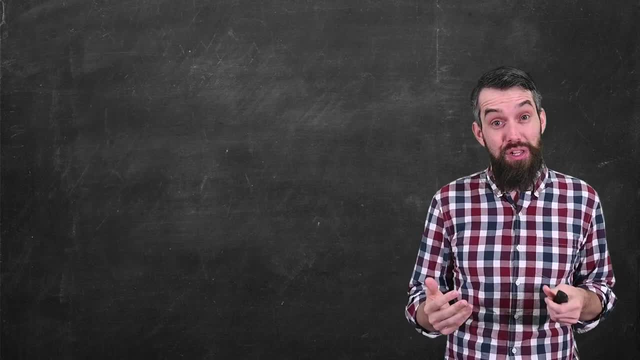 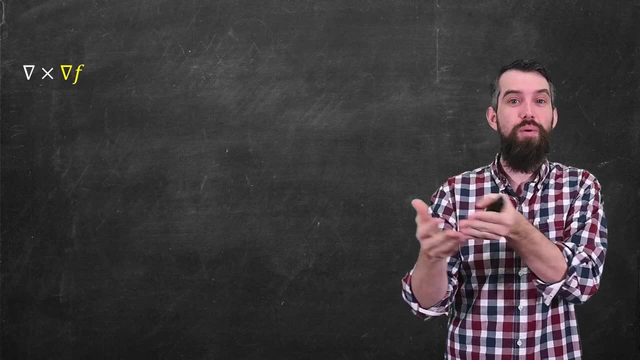 One last thing, playing around with the idea of curl, to specifically focus on, what is the curl of the gradient of f? Now, whether is del cross the gradient of f? Well, I mean, I can just write out what this determinant is, exactly as I said before, 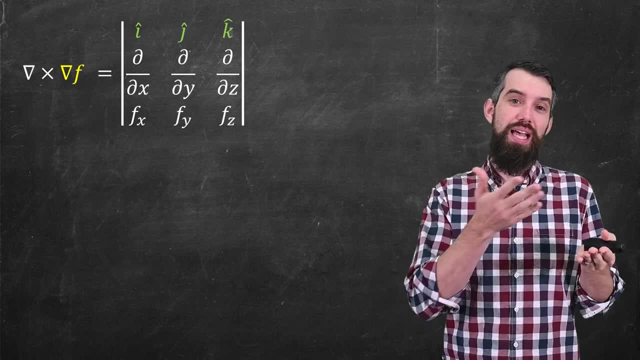 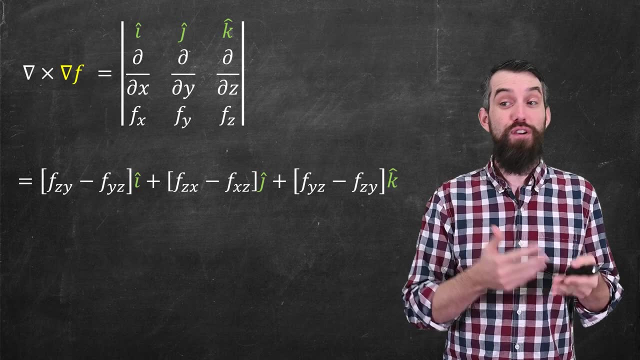 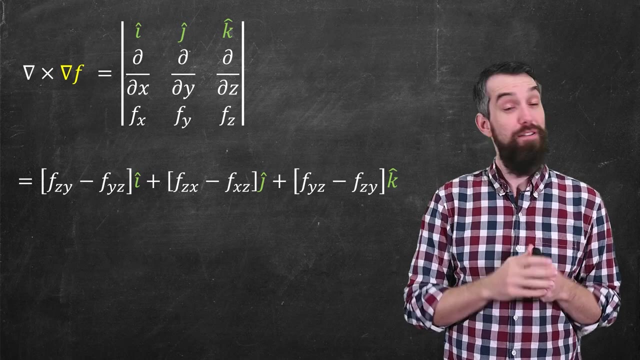 I can put the partials in the second line and the gradient of f has components fx, fy and fz in the third line. So executing this particular cross product, the first component, well, it's fzy minus fyz, As in the order of the partials have been computed. 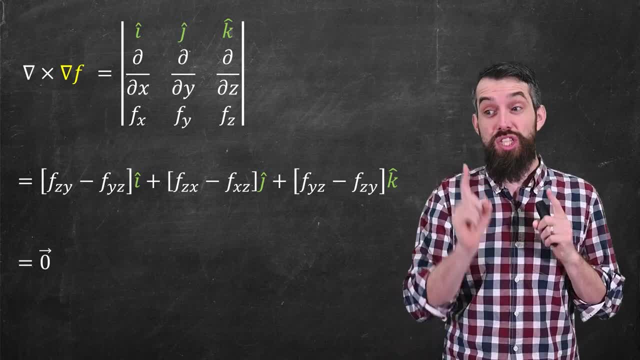 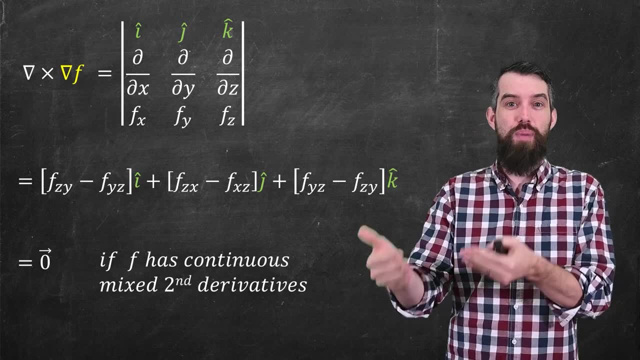 And in fact this is true for each component, And so, as a result, this is 0, provided you have some nice conditions on your f. For example, it has to have a continuous mixed second partial derivative. If that's the case, then the curl of the gradient of f is just 0. 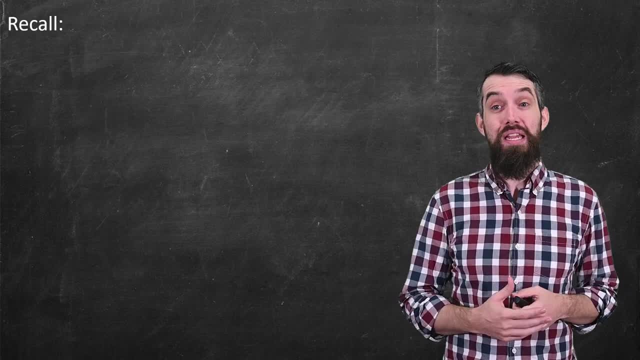 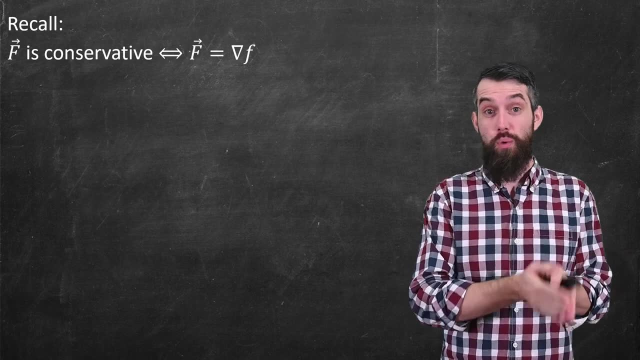 Now why is this so nice? Well, we've seen previously that the gradient of f was associated to conservative vector fields. So a vector field was conservative if it could be written as the gradient of f of a scalar potential function. And indeed conservative was a really nice property because 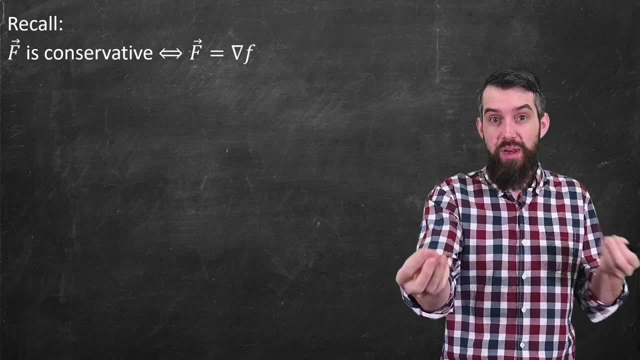 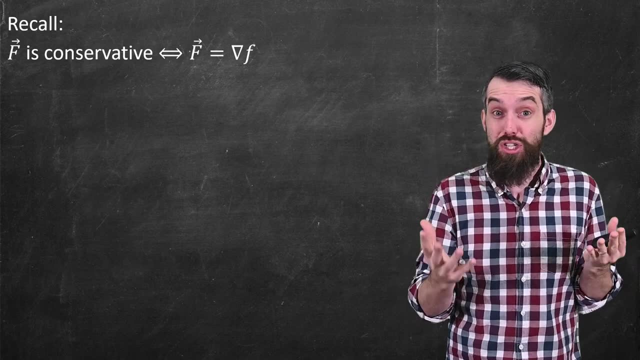 it meant that any line interval was independent of the path, only dependent on the endpoints. We had, for example, the fundamental theorem of line integrals. that only applied for conservative fields. Conservative fields are everywhere because things like, for example, the gravitational field, 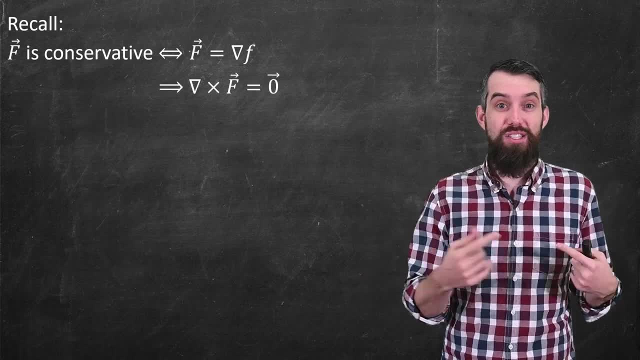 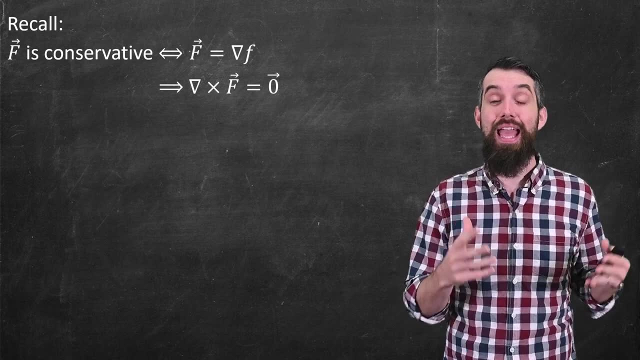 or the electric field are both conservative fields And so, because of the computation we just did, that showed that the curl was going to be zero if you had a field. that could be written as the gradient of f, aka conservative. So this means that these common fields, like the 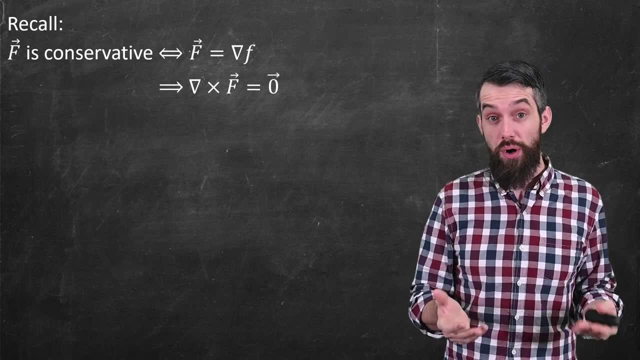 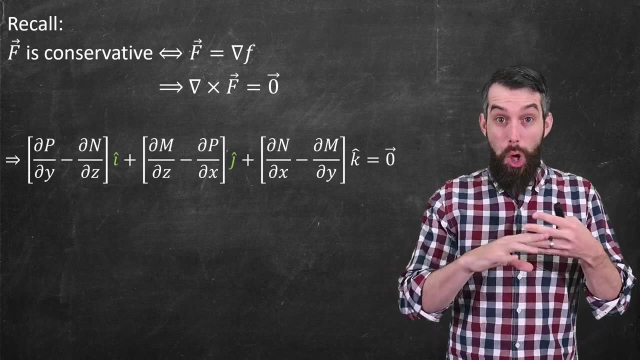 gravitation field or the electric field, these have no curl. And then I can also connect this to something we did back with conservative fields, because, okay, well, the definition that we've just seen was here's the longer version of what the curl is saying. that's equal to zero, But look. 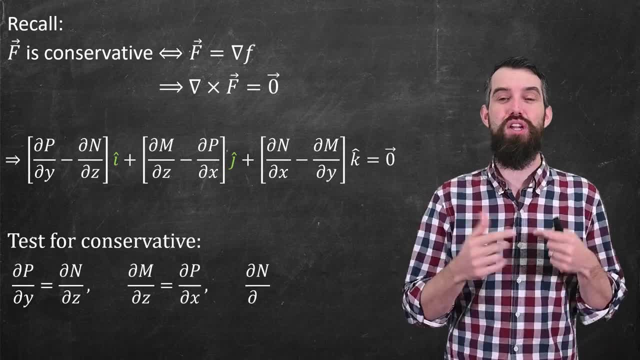 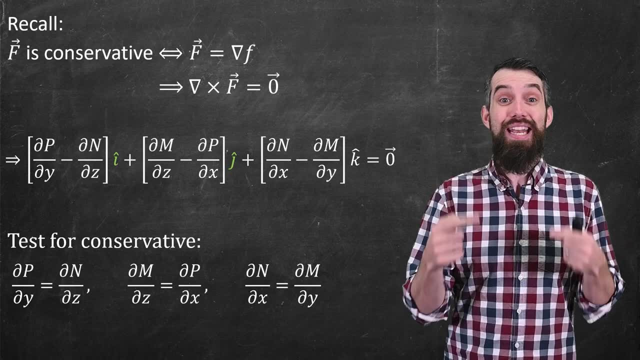 at those three components, You might recognize these. We had a test for conservativeness previously. It would say each of these three components had to be zero. In other words, the pair of partials have to be equals. So I can now.